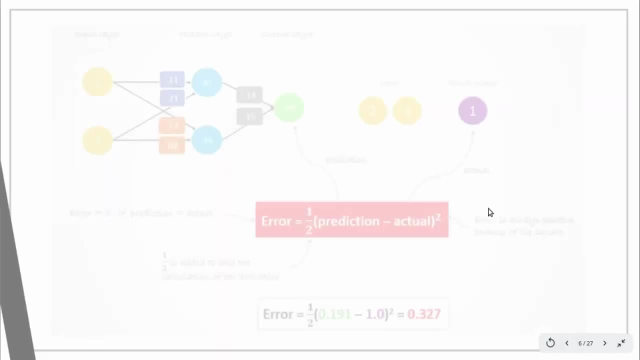 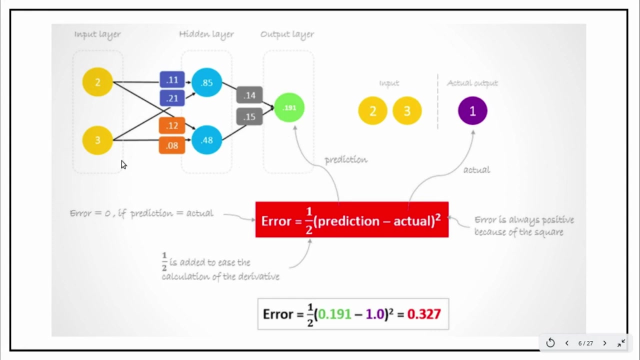 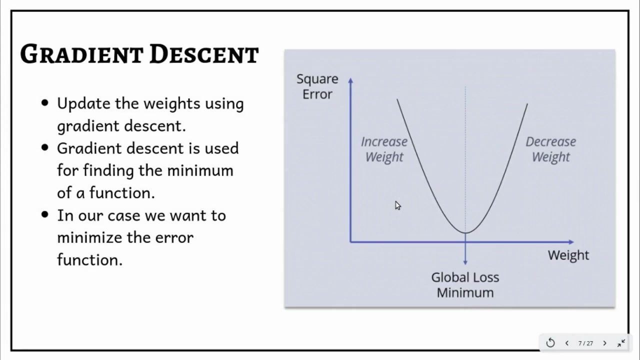 Now our model is way different than our actual output, and thus the error value is high. So what do we need to do? We need to somehow change this parameters such that error becomes minimum. And how we are gona do it? so lets introduce R好不好? So what? we are gona do it, So lets introduce R. 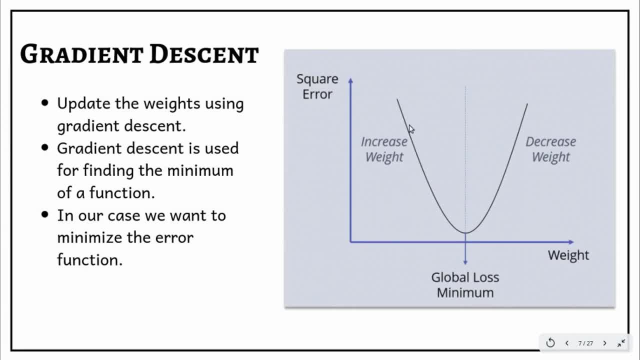 gradient descent. gradient descent method is used to update the weight by reducing the error function. so let's say at initially, if you were at this state, that is, the error was in this stage- then you will perform gradient descent. that is basically differentiation of this function and the slope will give you the direction where you have to go, whether you have to move. 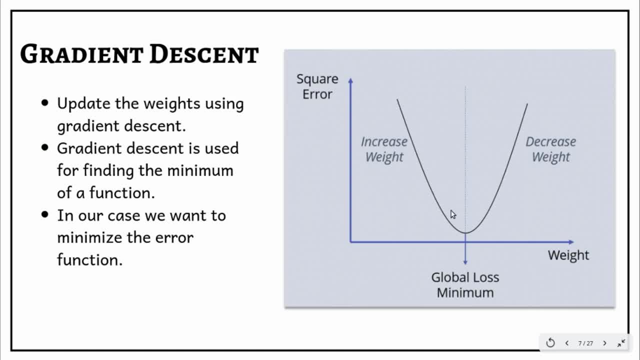 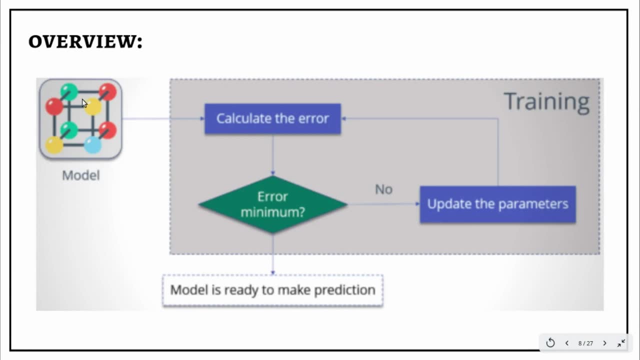 upward to reduce the error, or you have to go downward to reduce the error. so thus the gradient descent method helps to update the weight while also maintaining a minimum error function. so now let's understand the complete overview of backpropagation. so you have a model which we so we have a model that we will initialize with some random values. 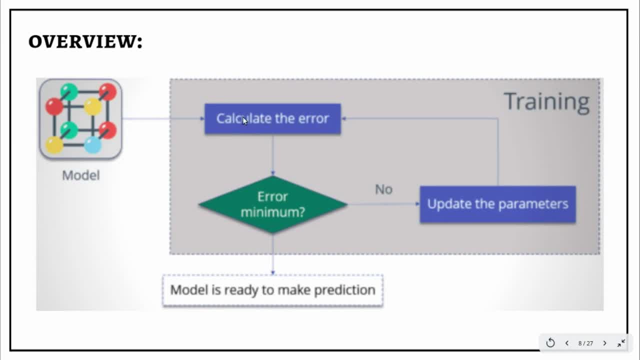 then at the first stage we will calculate the error that is, forward pass, and then we will calculate the error- actual output minus the predicted output. then we will see whether the error is minimum is or not. if it is minimum, then the model is ready to make prediction. 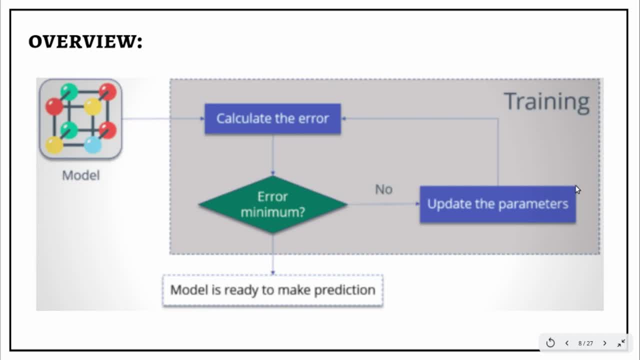 if it is not, then we have to update the pattern into method and then again we will calculate the error. again we will check whether the error is minimum or not, and this whole process is known as training the model. now let's understand backpropagation with a very simple example. 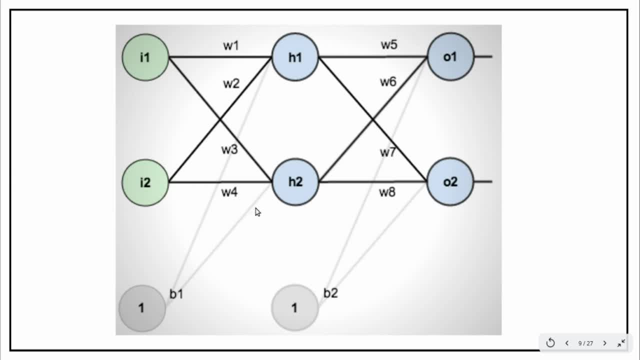 so here we are designing a neural network which has two input neurons, two hidden neurons and two output neurons. additionally, we are using two more things- that is known as bias- whose value is one which doesn't have any incoming node, but all it has is a value of. 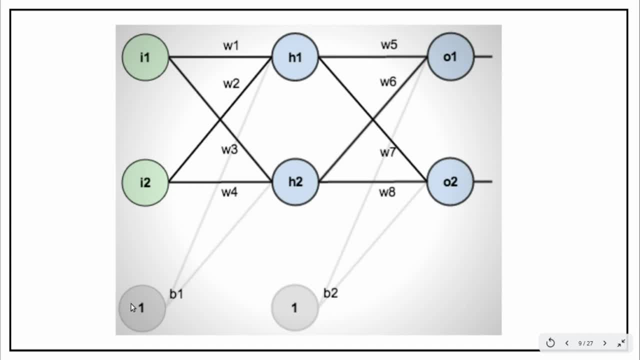 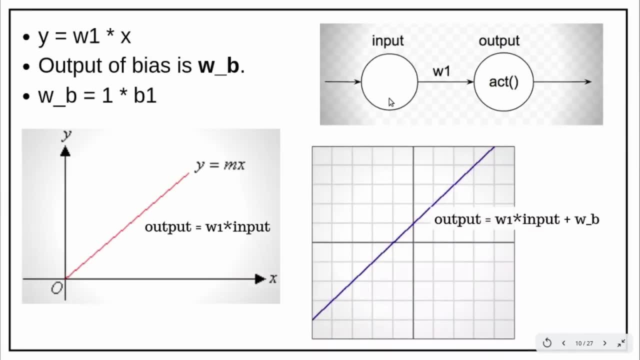 one which is an outgoing node. now a very important question arises: that why we are using bias when it doesn't have any incoming node and it is important to address it. so if i consider a very simple neural network that has only one input and one output, then obviously the 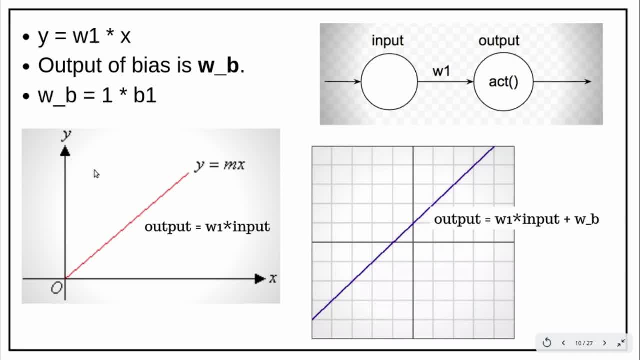 output of this neural network will be w1 into x. now if i plot a graph, then it will look like this: that is a straight line which always passes through origin. but what about the y intercept? in always, always, it will give the line which passes through origin. but there is a some possibility when we have to deal with y intercept. 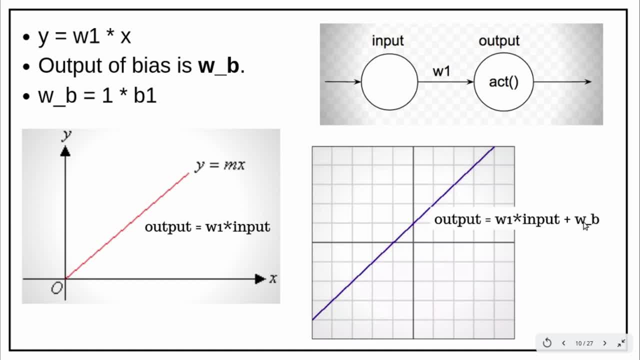 too. we have to use the output of bias, which is represented as w underscore b, whose value is one, into b1, where b1 is the weight of the bias. so this is what the main purpose of bias is. now, let's not get too much attached with it and should move on to our example, if you. 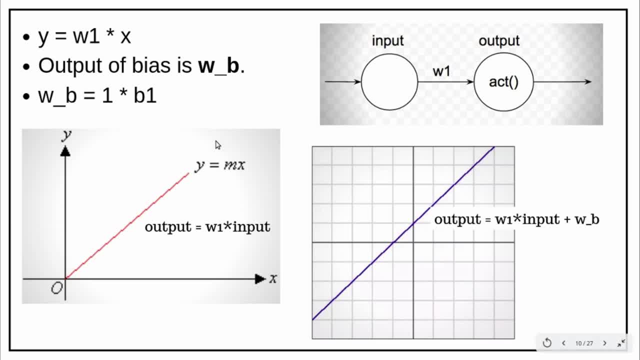 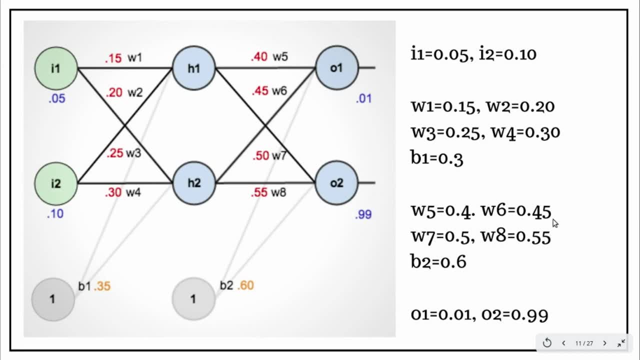 need more details about it, then you can find the link in the description to learn more. now this is the neural network which we were talking about. now all the values has been initialized, from i1 to i2 and from weight w1 to w8, and also the bias b1 and b2, and also. 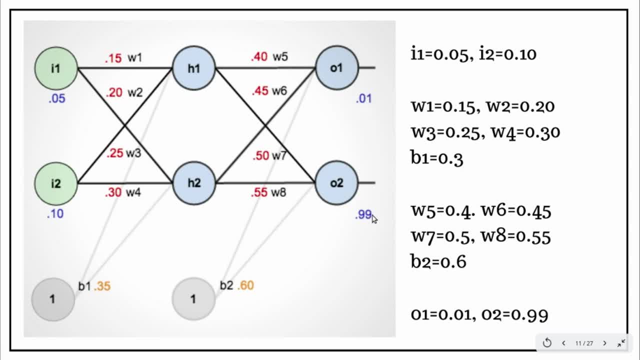 the actual output which we need, that is point zero one and point nine nine. here the first step is forward pass, that is, we will go from i1 to o1, that is, calculating our prediction output, by taking all this initialized or random values, then we will calculate the error that 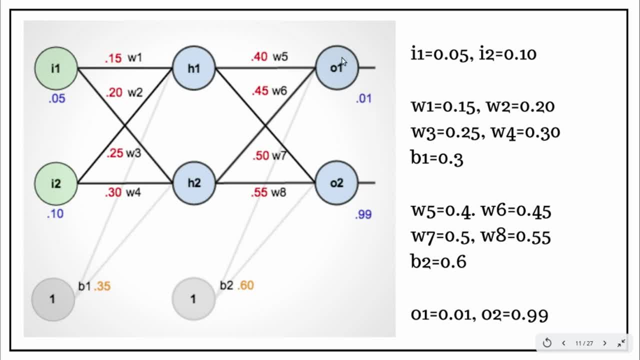 is the actual output minus the predicted output. and then we will move all the way back from o1 to i1 and update each values of this weights by using gradient descent method, such that the error should be minimum. again, we will go forward, pass, calculate the prediction output. 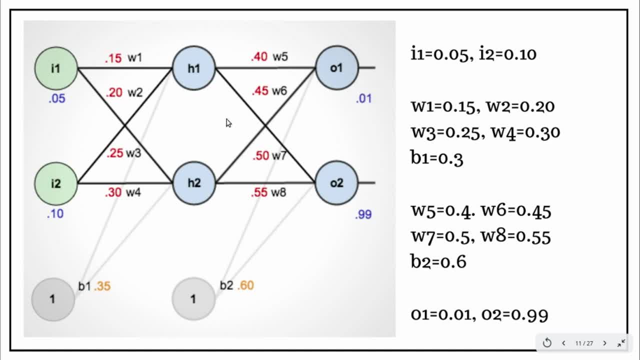 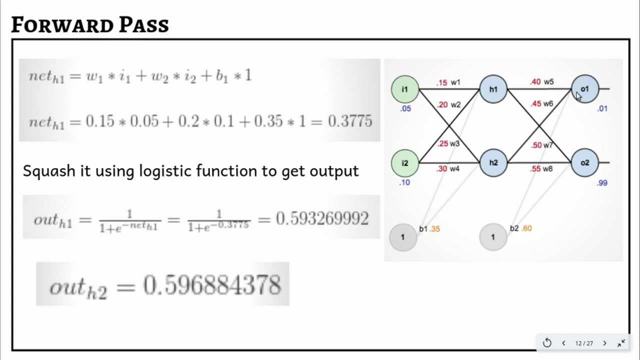 then we will calculate the error again, we will move backward and while updating all the weights, and the whole process will continue till the error is minimum. so let's see the first step, that is the forward pass. so what we need to do, we have to move from i1 to o1. so first of all we have to calculate the value of h1, that is net h1, so net h1 can. 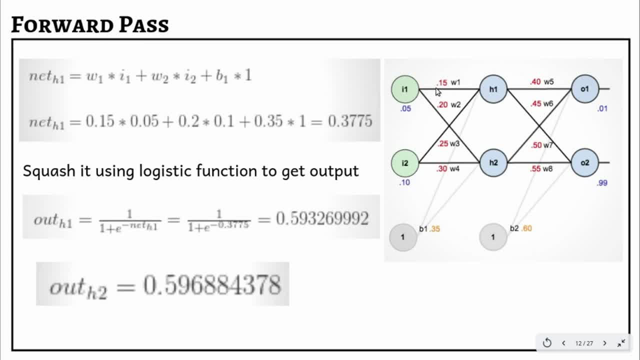 be calculated by seeing this lines you can see from h1 there is one line from i1 and one line from i2. so net h1 value and one line from b1. so net h1 value will be i1 into w1 plus i2 into w2 plus 1 into b1. that is what written over here. now substitute all the values. 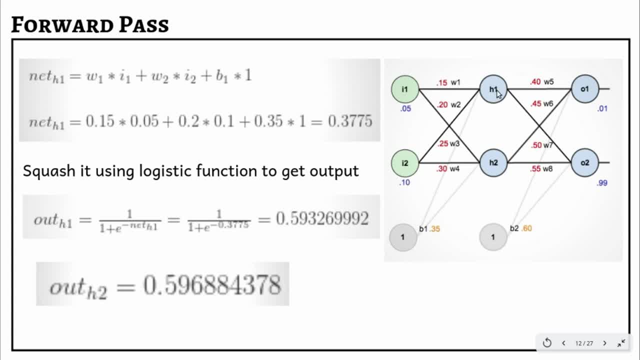 and you will get the value of net h1. similarly, you have to calculate the value of net h2. so net h2 will be i1 into w3 plus i2 into w4, plus- oh sorry- plus 1 into b1. that will be the value of net h2. but this net h1 and net h2 is not enough. you have to squash this function. 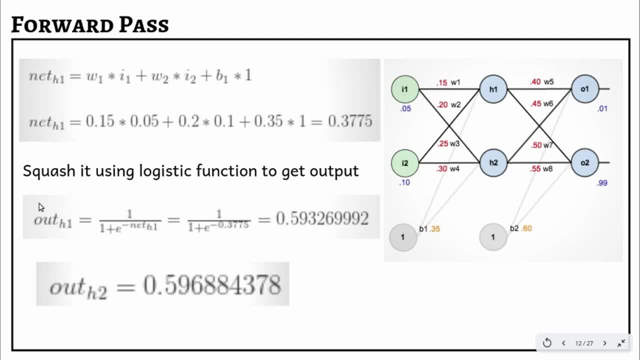 that is, you have to put the values between 0 to 1. thus for that you have to use this formula out: h1 is equal to 1 upon 1 plus e, to the power minus e to the power minus h1 as net h1.. So whatever net h1 you have calculated over here, just substitute its value and you will. 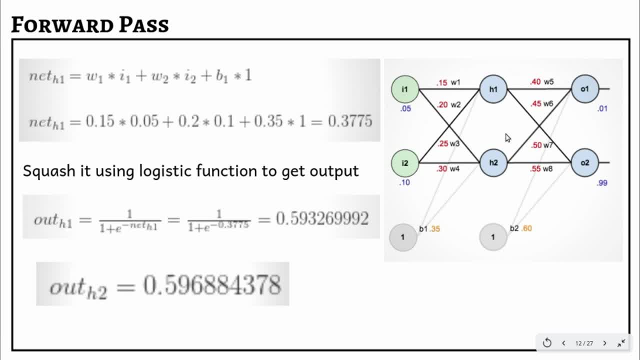 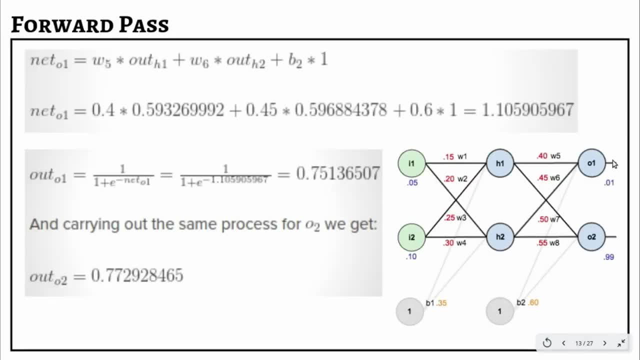 get the final answer of out h1, and same you have to do for out h2.. Now, since we have reached till h1 and h2, now we have to move on to o1 and o2.. So for o1 and o2, we have to follow the same. 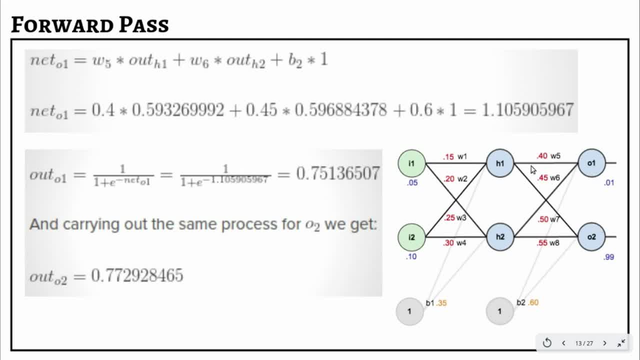 procedure: for o1, it will be h1 into w5 plus h2 into w6 plus 1 into b2, and similarly for o2, it will be h1 into w7, h2 into w8 and 1 into b2.. As we have calculated net o1 or net o2, now we will 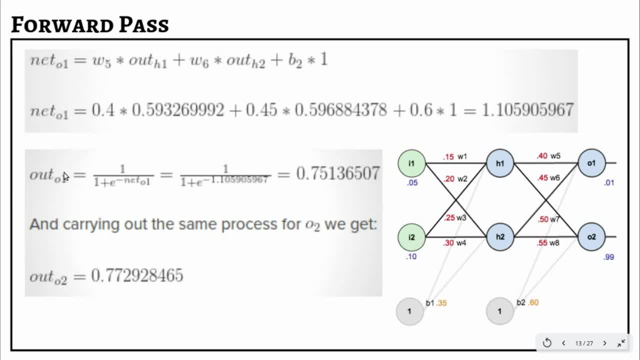 calculate out o1 and out o2.. So out o1 formula will be again the same thing: 1 upon 1 plus e to the power minus net o1. substitute this value and then you will get the output value. Similarly you have to perform this operation for out o2.. Now you can see our output value of first node. 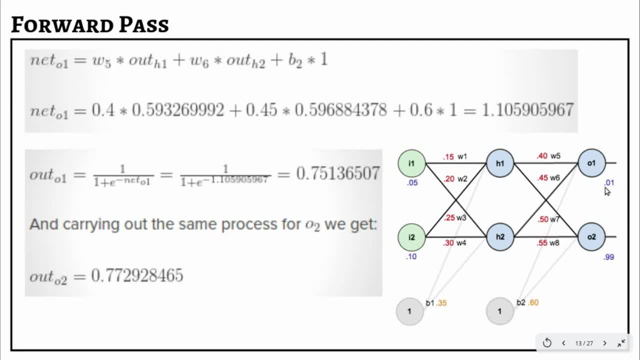 is 0.75, but what we need is 0.01.. And for second, the output value is 0.772, but what we need is 0.99.. So obviously there is a huge error. So what you have to do, you have to now calculate error. So how to calculate a error? 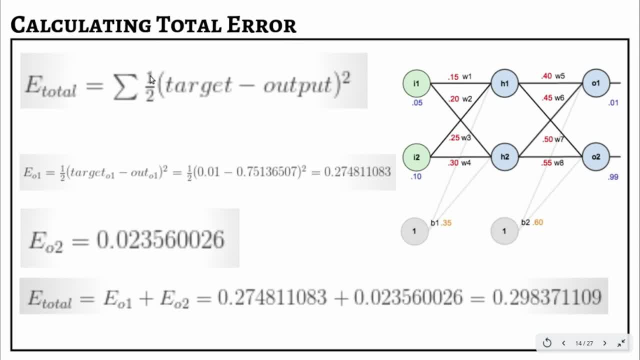 Error is defined as summation of half of target minus output. Here this target is the actual value and this output is the predicted output or the output which we were getting. So if I will calculate for o1, then half of what was the actual output, that is 0.01.. 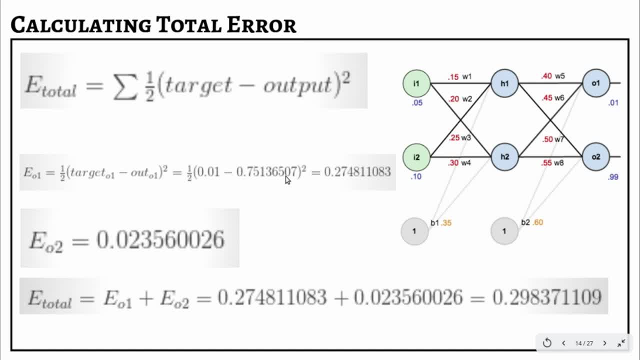 And what output I am getting. that is 0.75.. So this was the error for o1 and similarly I will calculate error for o2 and the total error will be e o1 plus e o2.. So this is my total final error. 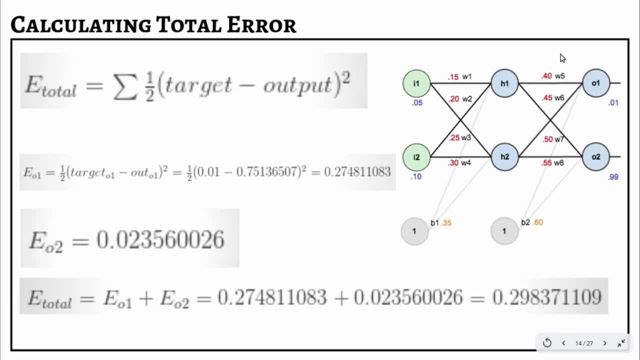 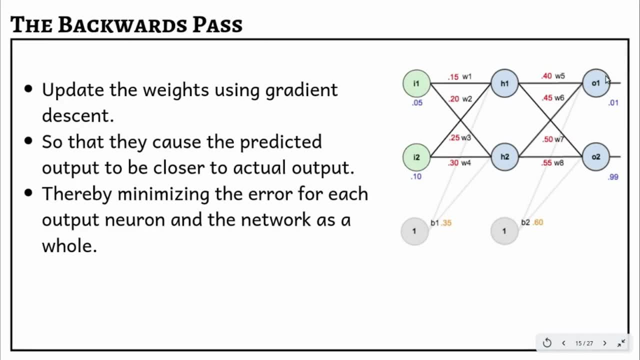 Now what we have to do. we have calculated the error. now we have to update the weight such that this error value should reduce. So we will go backward path, that is, we will move all the way from o1 to i1 and we will update each values such that our error should be minimum. 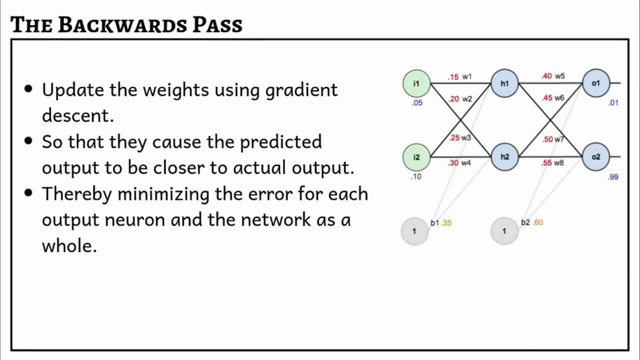 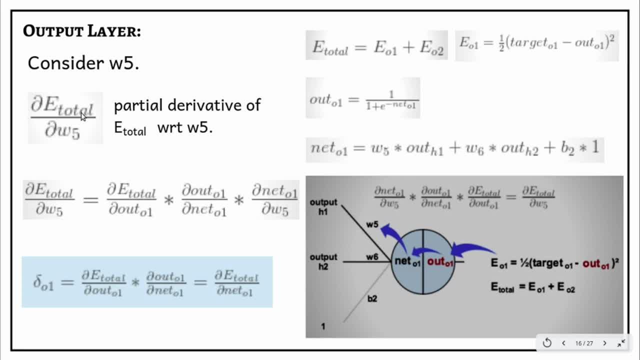 So from here on, I will suggest you to follow up with me, write it down so that you can understand the things thoroughly. So first of all, we will consider the weight, w5.. Now we have to calculate the partial derivative of total error with respect to w5. that is, you have to partially differentiate. 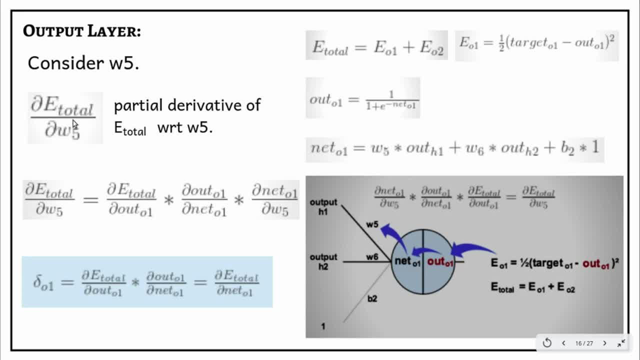 it, but you cannot directly differentiate it. you need to find some relation between this total error and w5.. So you have seen a lot of formulas before where e total is dependent on out o1 and this out o1 is dependent on net o1 and finally, net o1 is dependent on w5.. 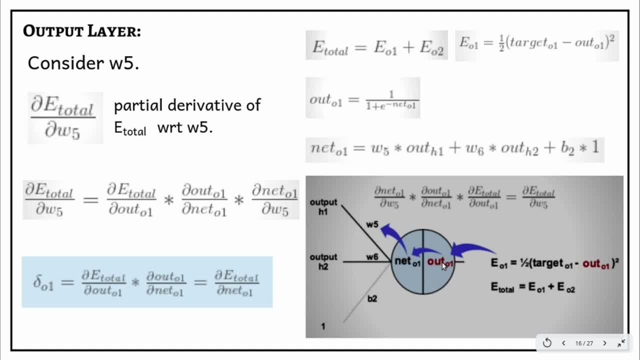 Diagrammatically it will look something like that: that the total error is now dependent on out o1, out o1 on net o1 and finally net o1 on w5. So we can write the formula directly over here. if you know homogeneous differentiation well, then you can understand it very clearly. So total error. 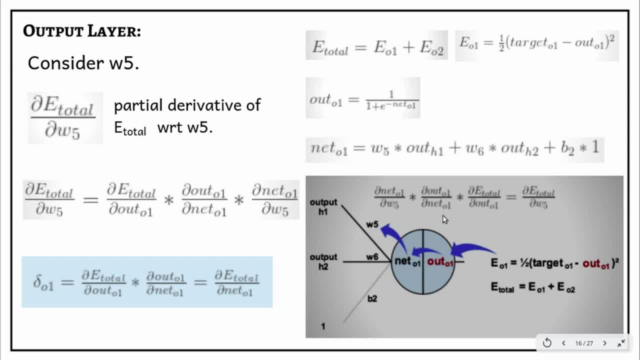 partial derivative of total error with respect to out o1, then out o1 with respect to net o1 and finally net o1 with respect to w5.. So this is what the formula which we have: derivative of total error with respect to w5. by using this- Now you have seen the first two terms- yeah, the 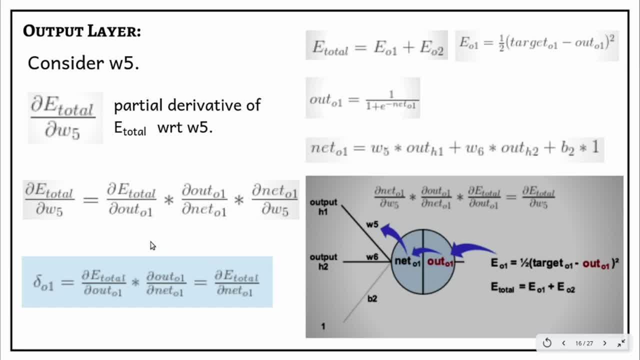 multiplication of these two terms is also known as delta rule or delta function. that is, the total error partial derivative of total error with respect to net o1, this is just the term which you might have heard before, or something like that. So now, just moving on, we will calculate. 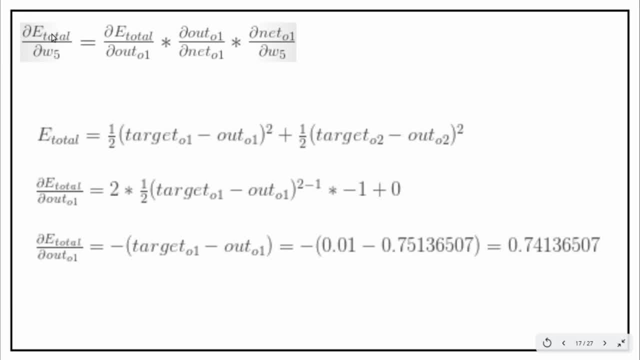 our partial derivative of total error with respect to w5 and we have got the formula. so we have to calculate the first term. so we know what is e total. e total is defined as this and now we have to differentiate it. so this particular last term, that is, the second term, will be treated as constant and the differentiation 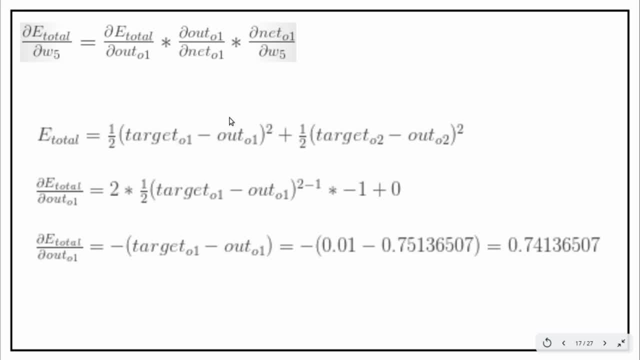 of this will be: and differentiation of the first term will be: 2 into 1 by 2. target of O1 minus out O1 to the power 2 minus 1. substitute all the values, you will get the value for partial derivative of total error with respect to out O1. so we have calculated the first term. now we have to calculate. 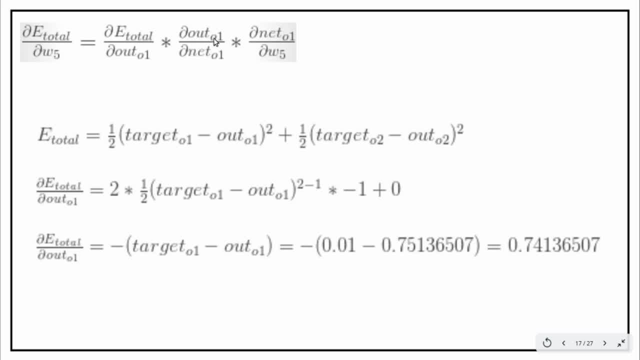 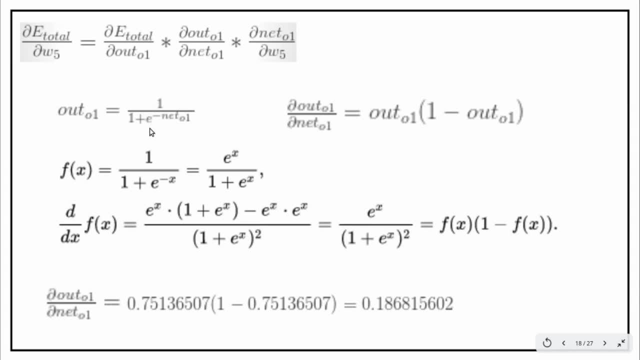 the second term, that is our partial derivative of out O1 with respect to net O1. so we know what is out O1. out O1 is 1 upon 1 plus e to the power, minus net O1. so if you will differentiate it partially, differentiate it with respect to net O1, then this is what the value we will. 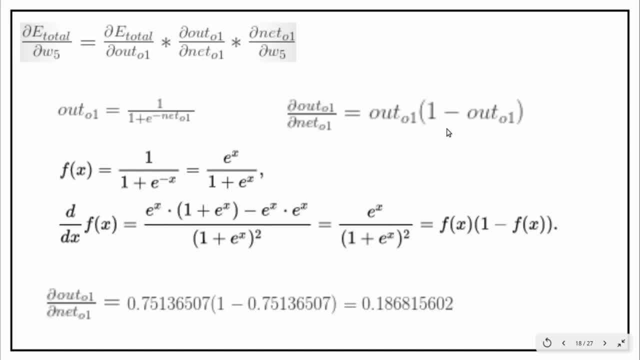 get. if you have any confusion with the differentiation, then look at this term: 1 upon 1 plus e to the power minus x. I am just replacing net O1 with x. now, if you will transform it, then e to the power minus x can be written as 1 upon e to the power x. and if you will further. 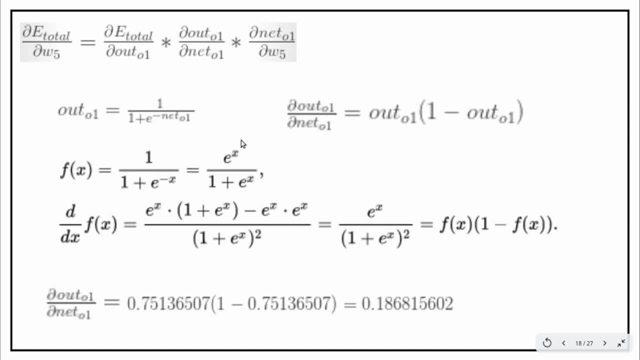 transform it, then it will become e to the power x upon 1 plus e to the power x. now it looks easy to differentiate it, so its differentiation will be e to the power x upon 1 plus e to the power x. So now, if you will split it into two terms, that is e to the power x upon 1 plus e, x multiply. 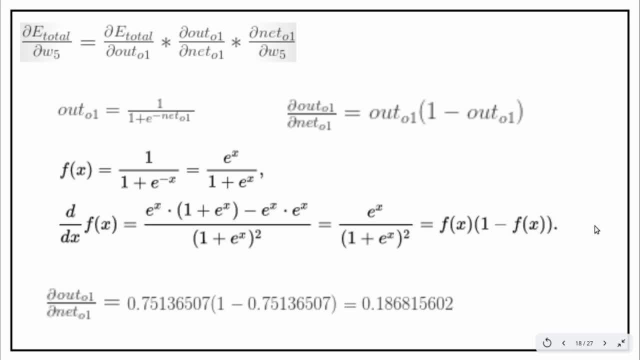 by 1 upon 1 plus e to the power x, then this term will be considered as f of x. you can match it, and the other term will be considered as 1 minus f of x. so like that we got the partial derivative of out O1 with respect to net O1. now substitute the values and you 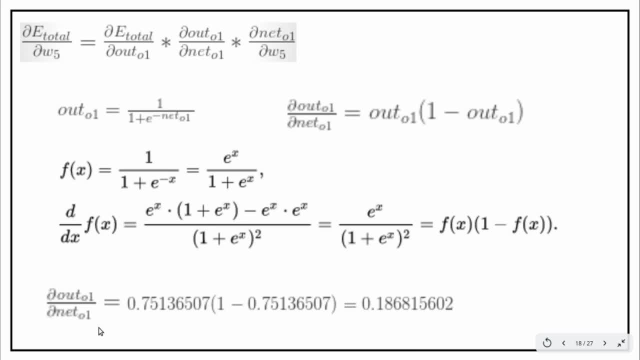 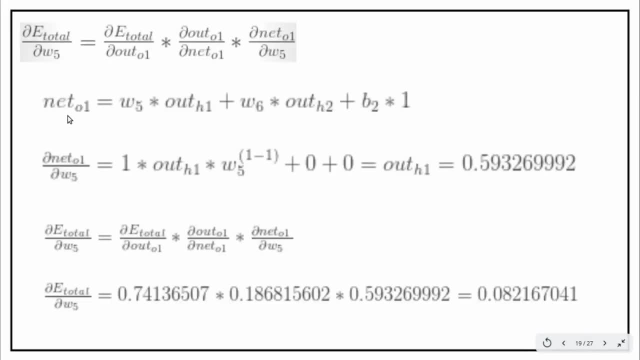 will get the final answer for out: O1 with respect to net O1. now we have calculated first two term. the last term is remaining net O1 with respect to W5. so when we will calculate it you know the formula of net O1. then we will differentiate it with respect to W5, then the 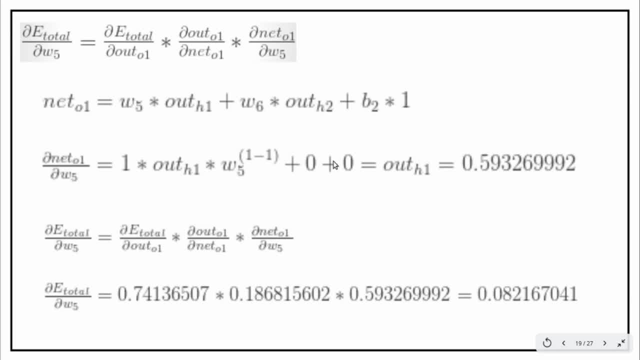 last two term will be considered as constant and its differentiation will be 0. and finally, we will get the answer as 0.5932. now we have calculated all the three values. substitute it and you will get the final total error with respect to W5. but still, we have just. 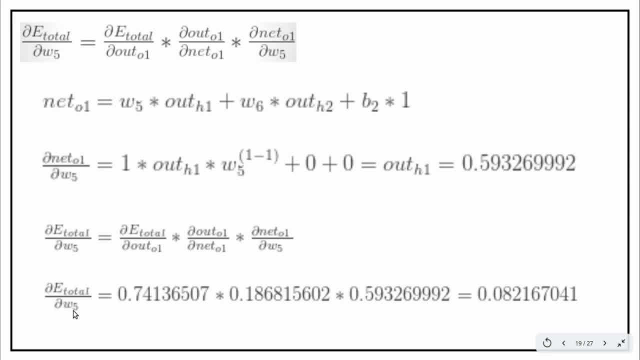 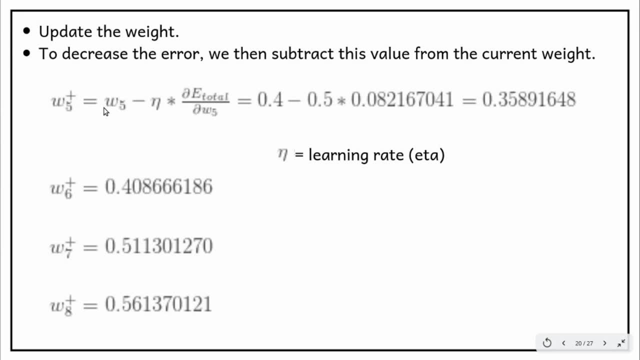 got the total error with respect to W5. we have to now update the weight. So to update the weight we have a formula that the final updated weight is equal to initial weight minus eta into total error with respect to W5. it is also known as gradient. 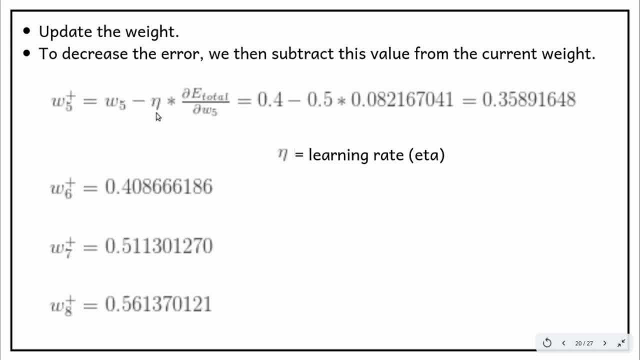 of W5. so what is eta? over here, eta is defined as the learning rate, which actually tells that how far you have to go, or what is the rate you want to increase your weight or decrease your weight, something like that. so here, what was the initial weight? initial weight was: 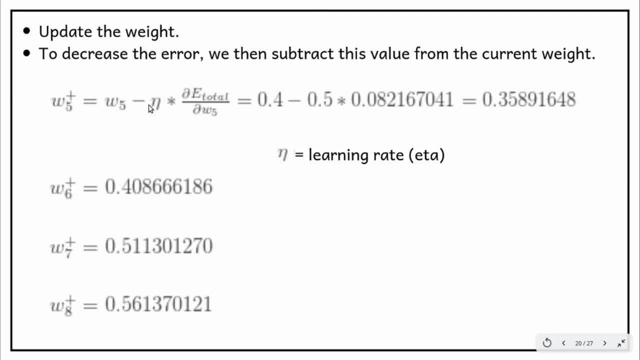 0.4 here. the value of eta I am considering as 0.5 and the total error which we have got. I have substituted the value over here and this is what the final error is, and this is what the final error is. So this is the final weight, the updated weight which we have got. similarly, we will perform. 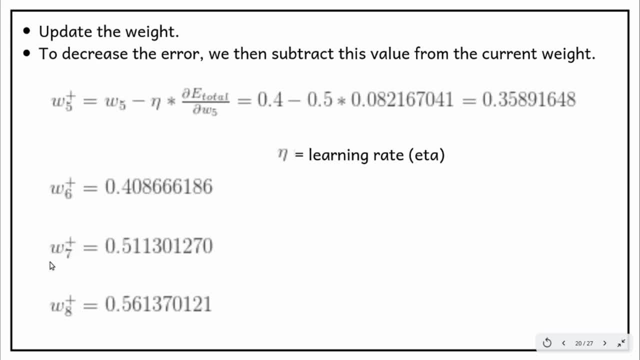 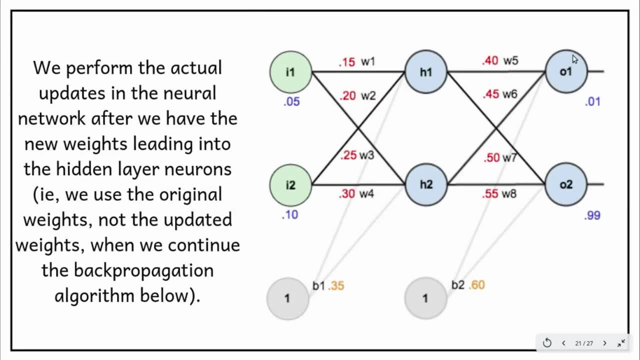 the operation for W6, W7 and W8 and we will get the final updated weight over here Now. since we have moved from O1 to H1 but we have not moved till I1, we are still here at the intermediate stage, so we will perform the actual updates in this weights only when. 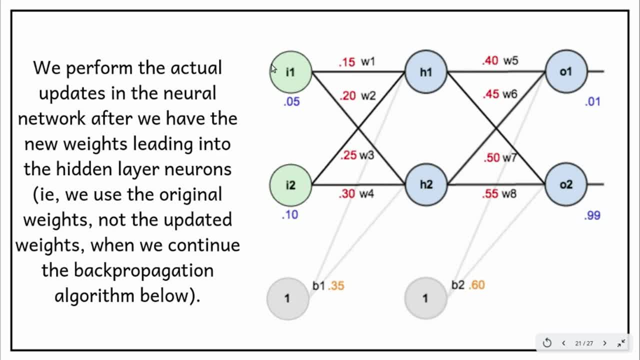 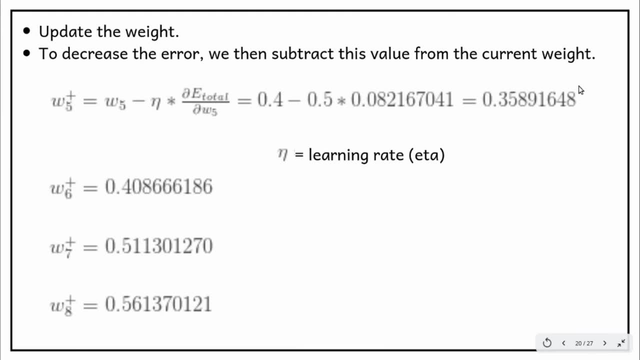 we have reached till I1. what I mean to say over here is: let's say, if I have to move from H1 to I1 and let's say if I have to use W5 in between, so I will use the initial weight, not this updated weight. are you getting what I mean? I am telling that if I have to use 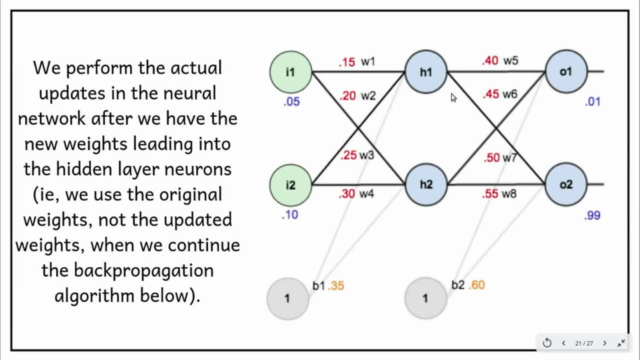 W5 at this stage, then I will not use the updated weight W5, but I will use the initial weight which I have used. So now we have to move from H1 to I1, so again that we have to calculate first of all. I am 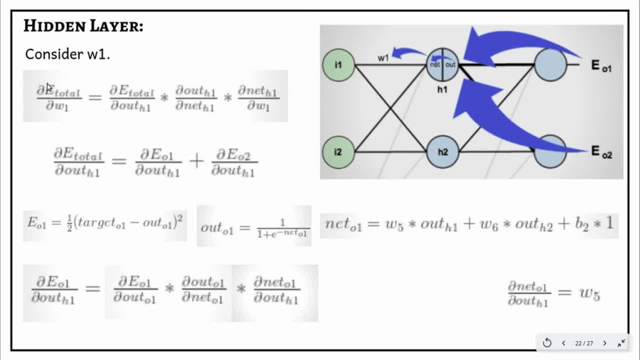 considering W1.. So we have to calculate the partial derivative of total error with respect to W1 and it will be equals to E total divided by out H1. you can see how it is dependent: EO1 on out H1, out H1 on net H1 and then net H1 on W1. but still there is a confusion with E total by. 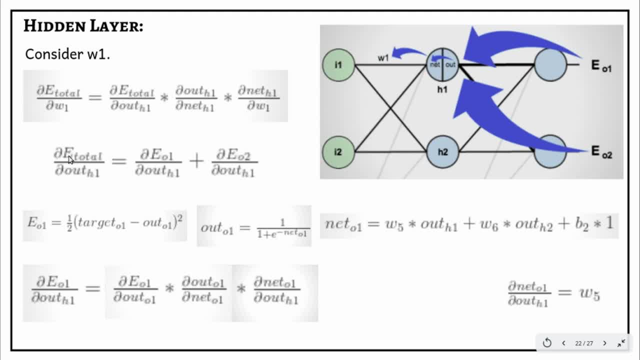 out H1 how it is related. so you can see E total by out H1 can be written as the EO1 plus EO2 and you know EO1 is dependent on out O1. out O1 is dependent on net O1 and this time net O1 is dependent on out H1.. 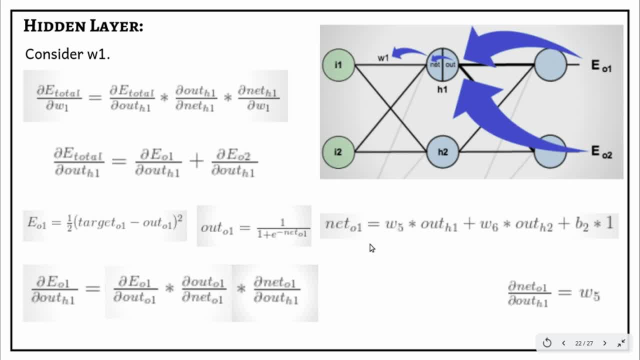 We will not see W5, but we will see out H1. why? because we need out H1. we need to find the relation between total error and out H1.. So now, if you will see the value of this first term, that is, EO1, by out H1, so it will something. 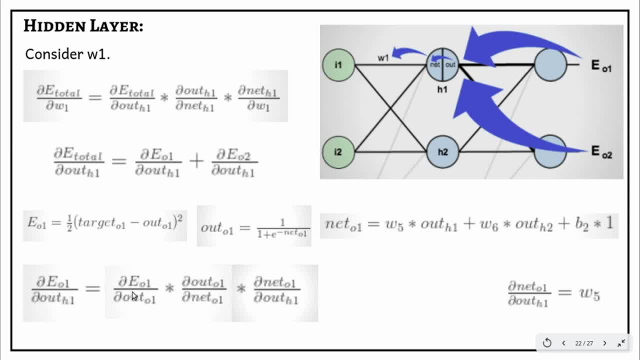 look like. it will look something like that: EO1 by out O1 multiplied by out O1 by net O1, multiplied by net O1 by out H1. so these two terms which we have already calculated before the last term, the differentiation of net O1 with respect to out H1 will be equals. 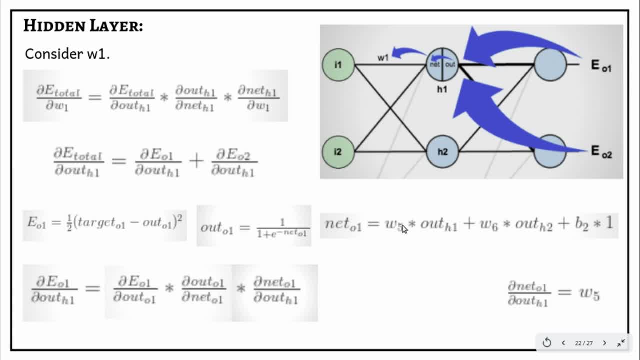 to W5.. So if we differentiate this with respect to out H1, then only W5 will be there. these two terms will be treated as constant and the differentiation will be 0.. So we have got the values for these two terms. substitute it, you will get the final answer. 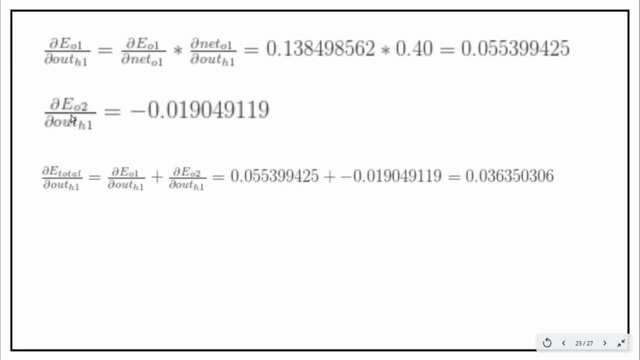 similarly, we will calculate for EO2 with respect to out H1 in the same way. now add both the terms so you will get the total error with respect to out H1. but still, we have just calculated the first term. we have to still calculate other two terms. so you know what is the formula. 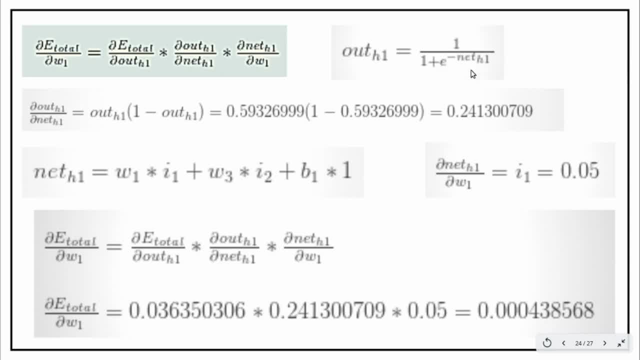 of out H1.. Out H1 is 1 upon 1 plus e to the power of 1, plus e to the power of 1 plus e to the power of 1.. Out H1 is 1 minus net H1. if you will differentiate it, then this is what the value you will get. 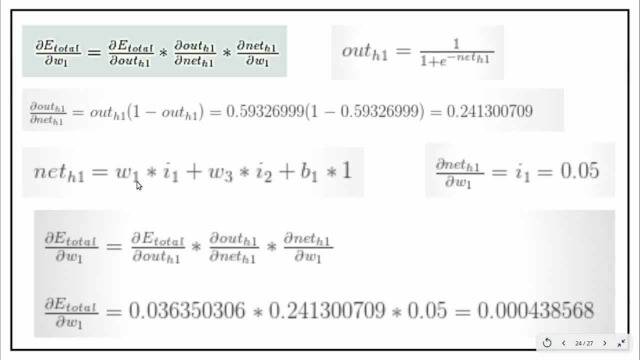 similarly for net H1. net H1 is W1 into I1, plus W3 into I2, plus B1 into 1. if you will partially differentiate it with respect to W1, then these two terms constant. it will become 0 and the final answer will be I1, that is, 0.05.. 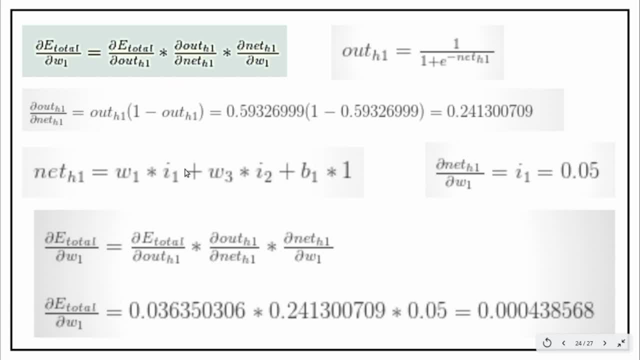 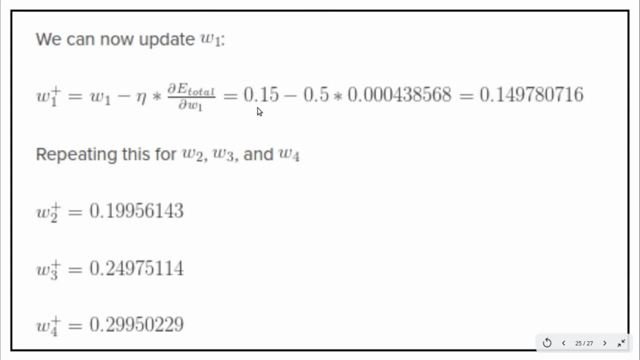 So now you have got value of all these three terms, substitute it and we will get the total error with respect to W1. now again we have to update the weight W1, so W1 is equals to 0.05.. W1 minus eta into total error with respect to W1. now substitute all the values as I have. 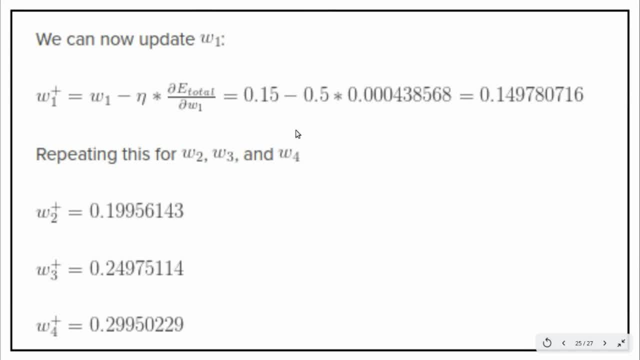 said, eta is the learning rate and the value is 0.5. substitute the values and you will get the final updated weight of W1. repeat this procedure, same for W2, W3 and W4. now, finally, we have updated all our weights when we feed forward the 0.05 and 0.1 inputs originally. 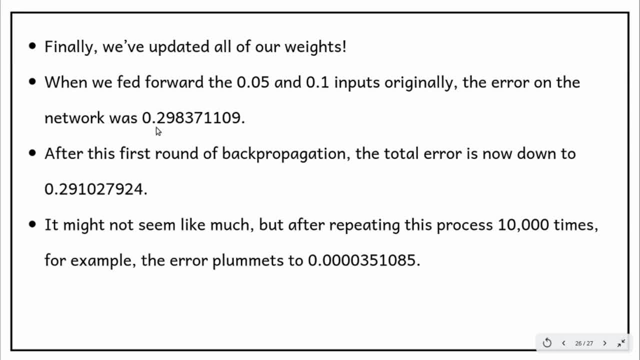 the error on the networks was 0.298371109 and after the first round of back propagation the total is now down to 29102. so yeah, there is a little change. what I mean to say here is: at the initial stage we have this error. now, when we have updated the weight after, 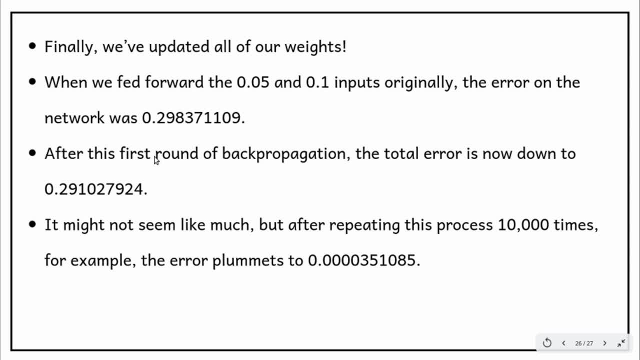 that we have got this much error, so there is a little reduction. if you will perform it for 10,000 times, then after that the error will be reduced to 0.000035. so this is how the back propagation helps. this is the entire process of back propagation. hope you have. 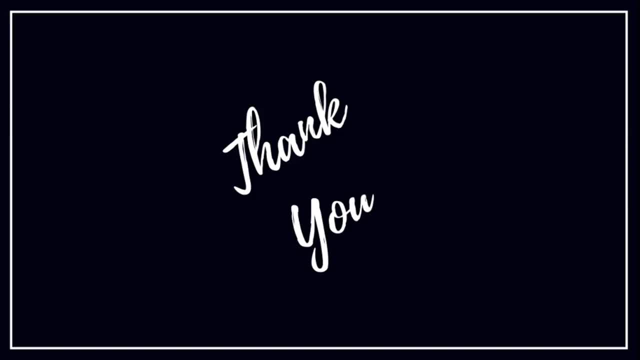 understood the video. Stay tuned with us. Do like us, Subscribe, share and comment. you can also write us at codewrestling at richgmailcom. so happy learning, thank you.